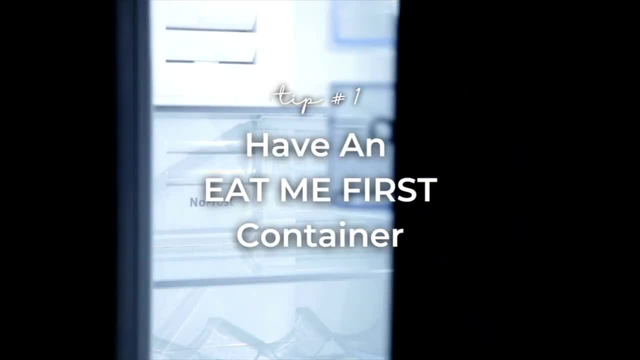 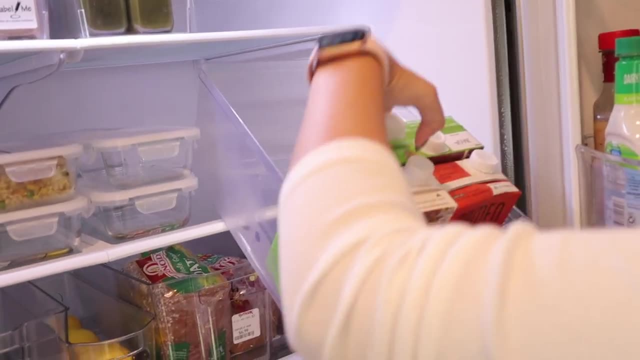 balconygardenwebcom, and it is to have an eat-me-first container for all the food that's going to expire soon. I love how it puts the focus on the items that need to be eaten before they expire and it reminds me to try to incorporate them. 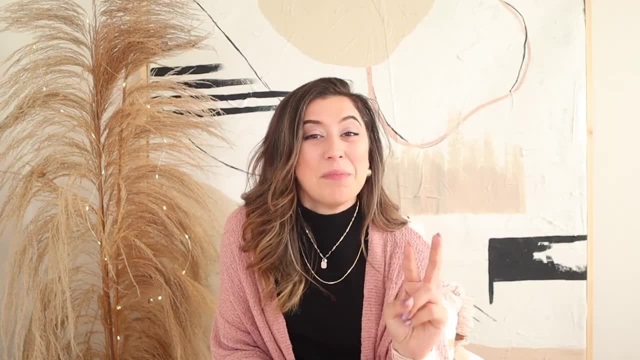 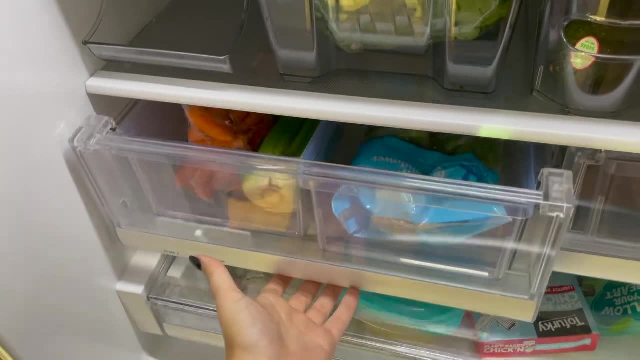 into the food that's going to expire soon. I love how it puts the focus on the items that need to be into my meals before anything else. Super smart. Tip number two I learned from realsimplecom, which was to use crisper bins or drawers. Supposedly, the fruit and veggies can circulate. 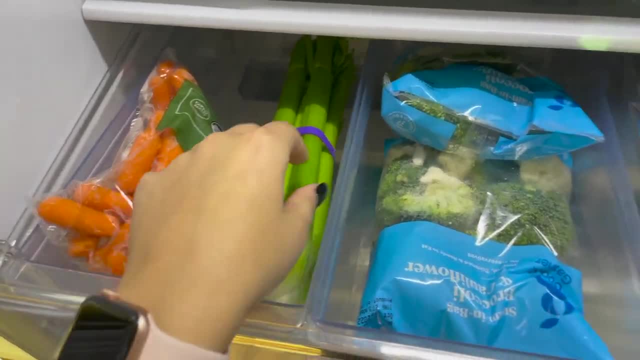 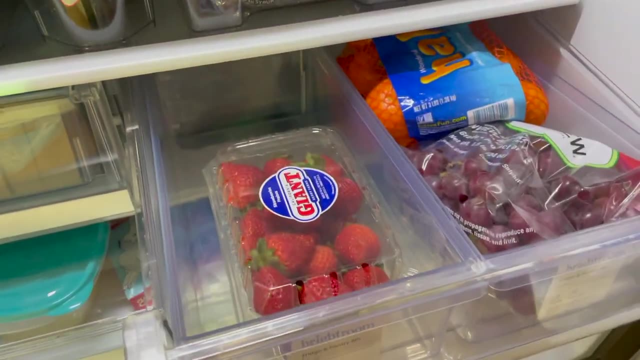 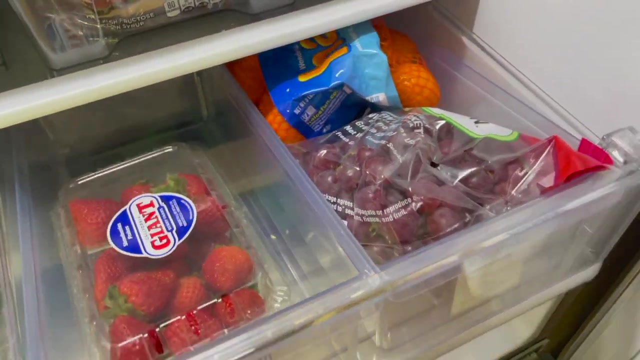 air and not get so crummy at the bottom in crisper bins. And after reading more about these bins I realized that our fridges, or at least most, come with the crisper drawers built in for your fruits and veggies to balance humidity: Vegetables last best in high humidity and fruits in low humidity. 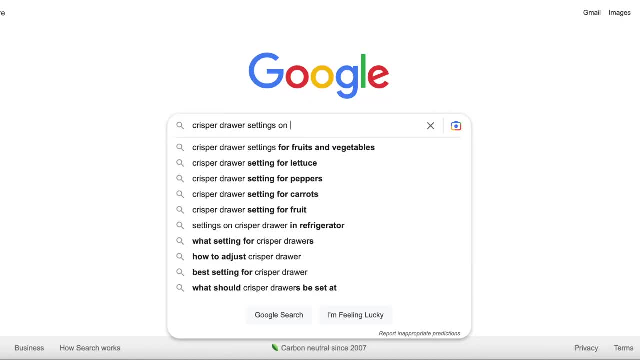 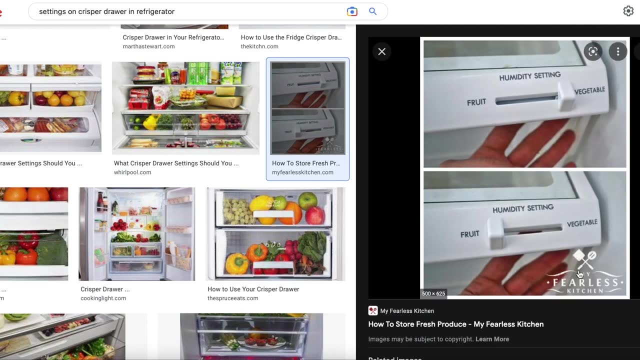 Most fridges will have settings on the crisper drawers to adjust the level of ventilation. If your fridge does not have these drawers, you can also buy these crisper bins individually, Because I learned so much from that article about crispers and vegetables. 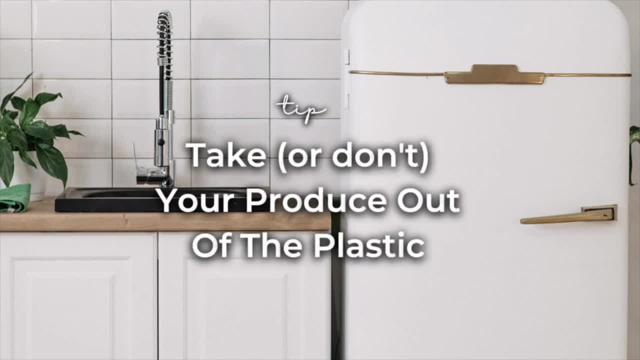 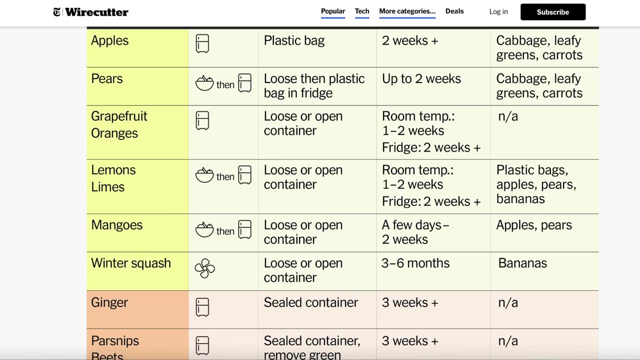 tip number three is to take, or don't take, your vegetables out of the plastic when you come home. This varies on the produce, but wirecuttercom had a really handy chart that showed which produce should be removed from their original container or not. If you do this, consider how you want to. 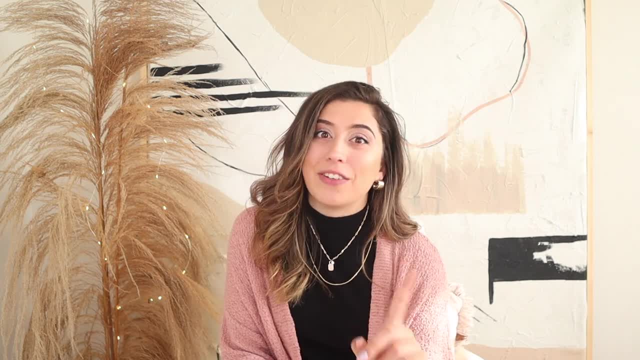 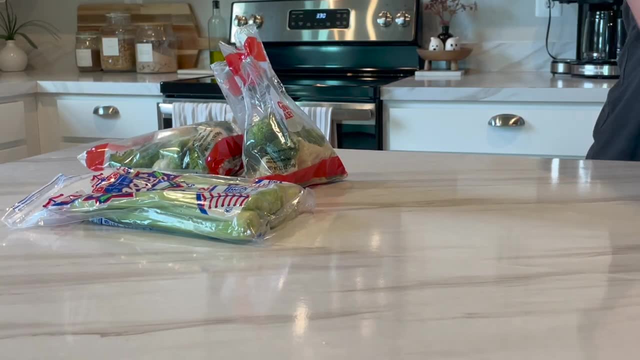 organize your vegetables, especially if they are touching and affect the flavors and or ripening of nearby veggies. And in all my research on produce and fridge organization I also realized I was contributing poorly to the carbon footprint by all of my plastic use and probably should do a better. 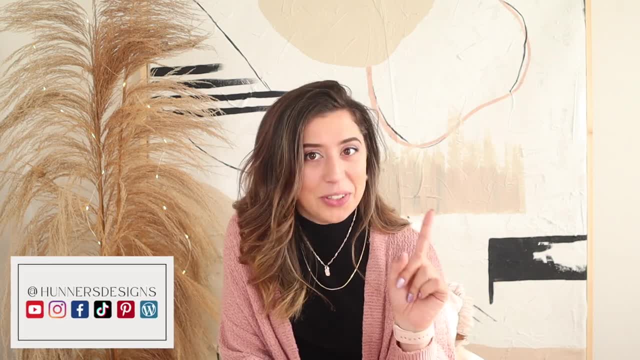 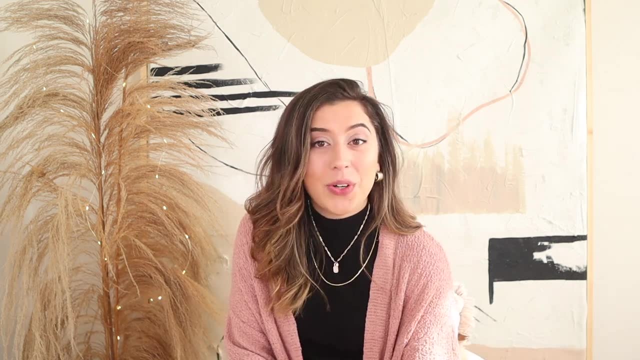 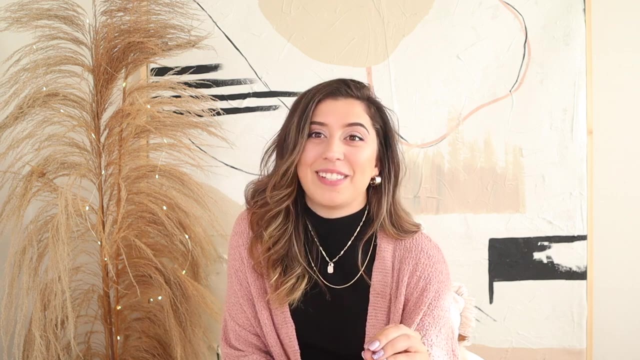 job at visiting farmers markets and things like that, So keep that in mind too. Tip number four is from hellonutrariancom, And personally I read this entire article. In this article, I learned about meal prepping your food first and then organizing it in the fridge. This makes the most sense to me. We're more of 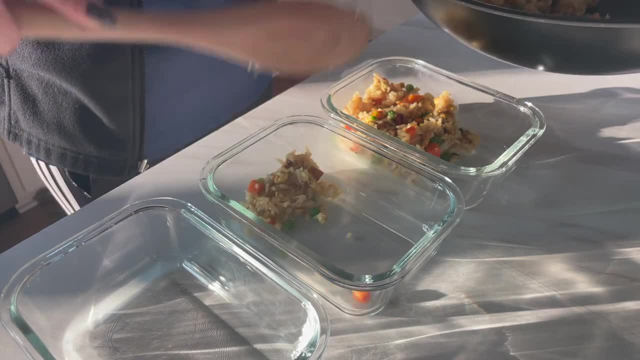 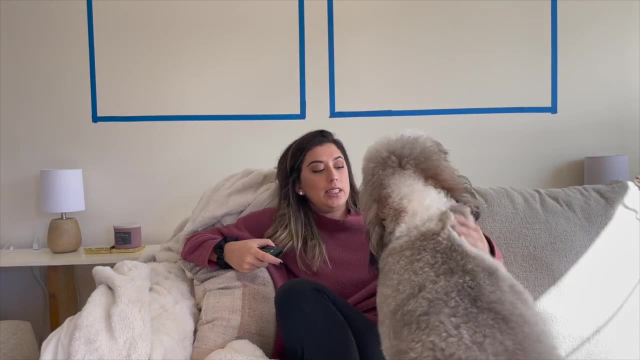 a meal prepping family. There's no cooking during the week. like incredibly time savvy people do okay During the week. we are working, gyming, TV, watching people- So I love the idea of sorting meals out into containers, then organizing those meals in the fridge, versus organizing ingredients. 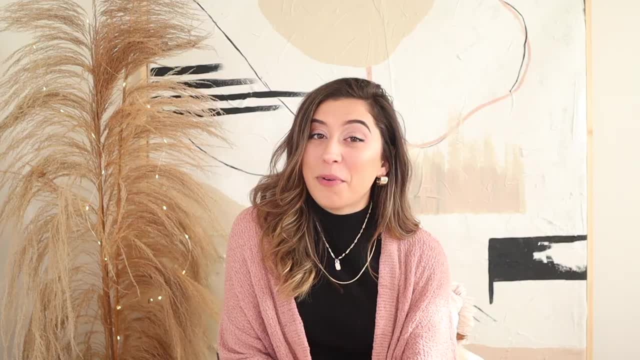 and not leaving space for leftovers, meals, etc. Tip number five is to have matching containers or bins for your fridge when you come home. Tip number six is to have matching containers or bins for your fridge when you come home. Tip number seven is to have matching containers or bins for your fridge. 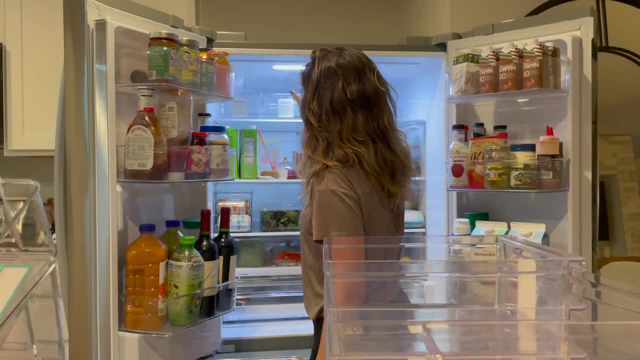 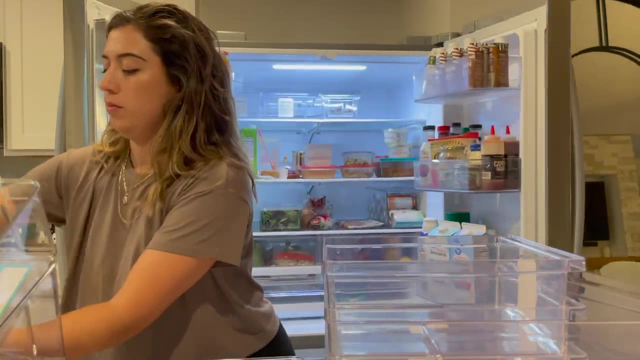 organization, namely glass or fridge freezer friendly ones. I'll link some of my favorites below. This just helps the fridge look so good And I know people watching this video care about that kind of stuff. Tip number six is to either plan which organizers you'll buy ahead of time. 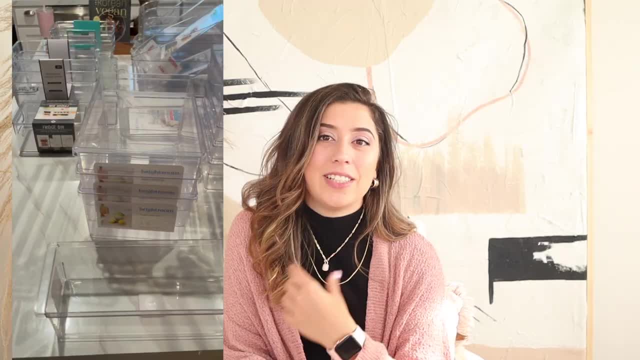 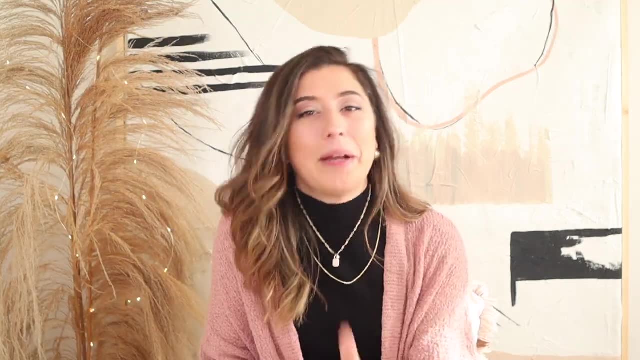 for your fridge organizing extravaganza, or do what I did and just buy an excess amount of them, so you have options when organizing. I also do this for my decor planning. by the way, The first thing I did was experiment with different container sizes in my 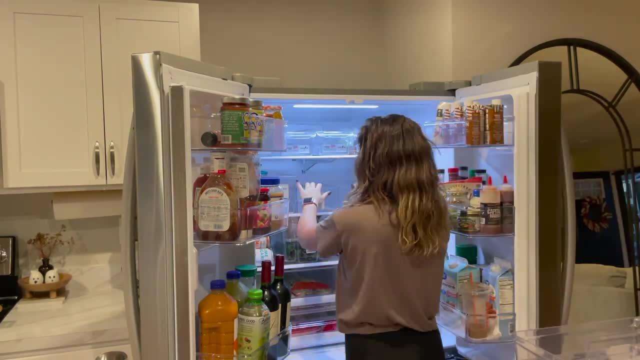 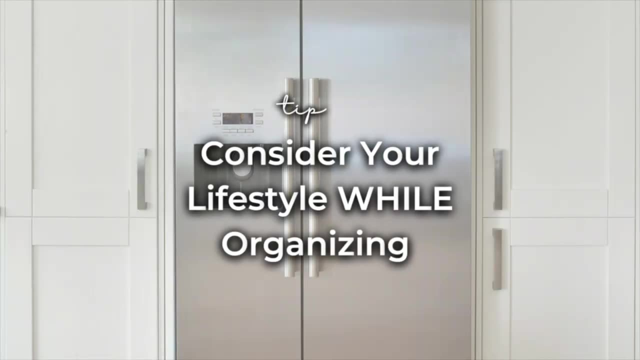 fridge to see which sections I could carve out and which sizes I preferred, based on our needs. Which leads me to tip number seven, which is to consider your lifestyle. For example, I remember that John and I go out to eat at least once a week and we usually have those. 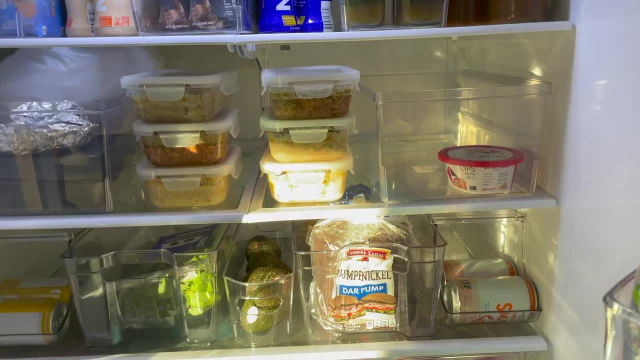 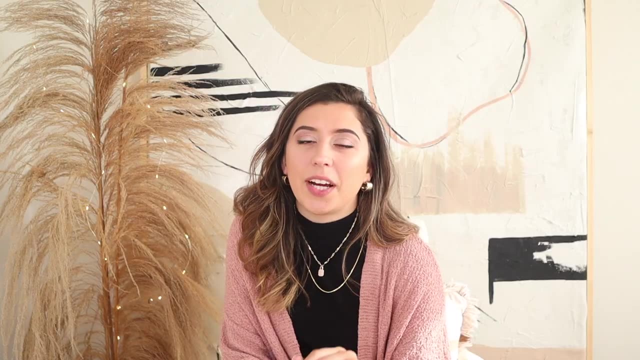 square styrofoam to-go boxes. So when I was planning out my fridge containers, I thought having a bin wide enough for these to-go boxes would be perfect. So don't forget to consider your lifestyle. Tip number eight is to separate your juices. 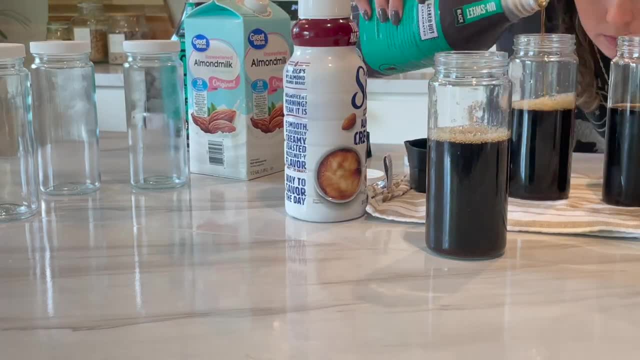 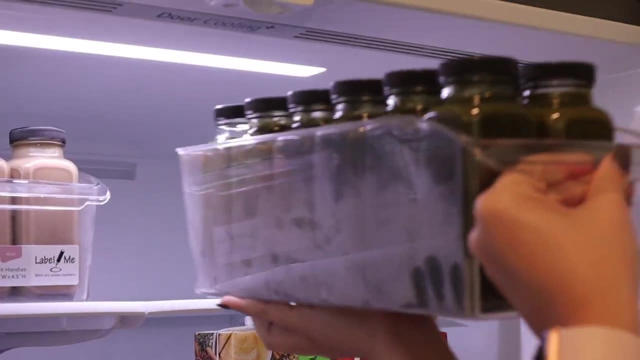 or other large containers of liquid into smaller jars. I got these jars on Amazon that fit perfectly on the top shelf. I got both eight ounce jars for juices and 16 ounce jars for things like coffee or flavored water. These jars are also pretty handy if we're making our own dressings. 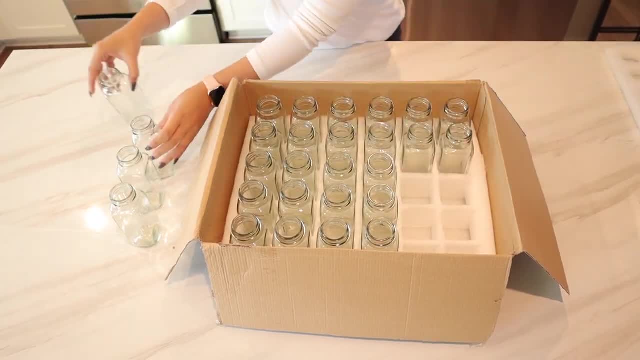 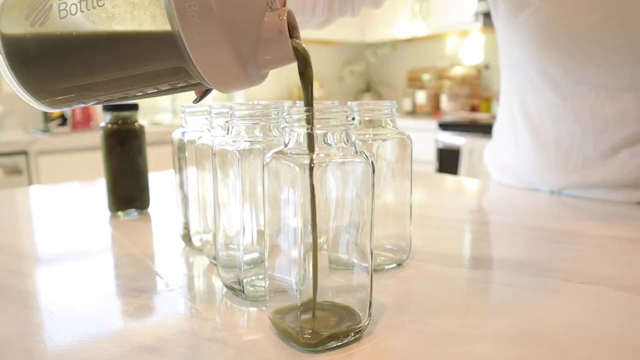 or sauces, or if we wanted to send some beverages with our guests home, such as apple cider, during the holidays. Overall, I feel like sorting out the liquids promotes us drinking them versus having the large bottle, just kind of like sitting there and taking all that space, And they're great for on-the-go. Now, before I move on to the next tip, 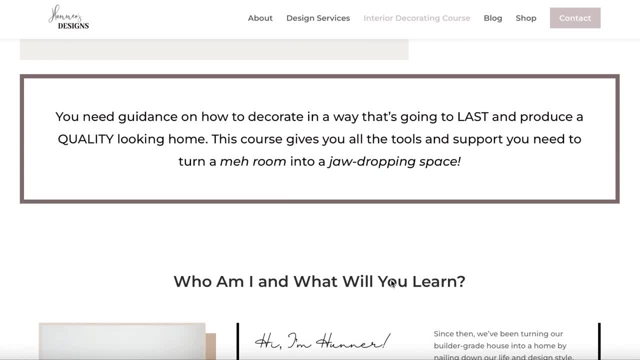 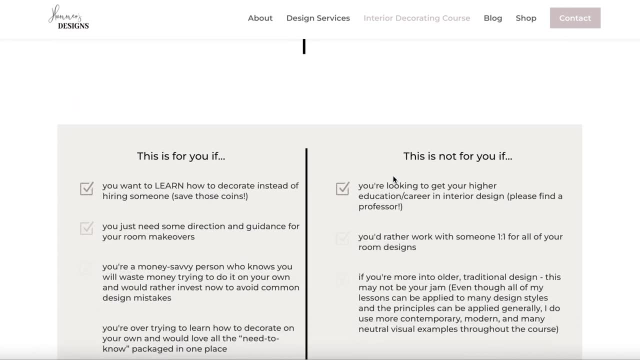 if you want to learn more about decorating and organizing your home, then make sure you check out my course in the description box and the comments section below. My course dives deeper in how to define your life and design style, how to plan your home design. 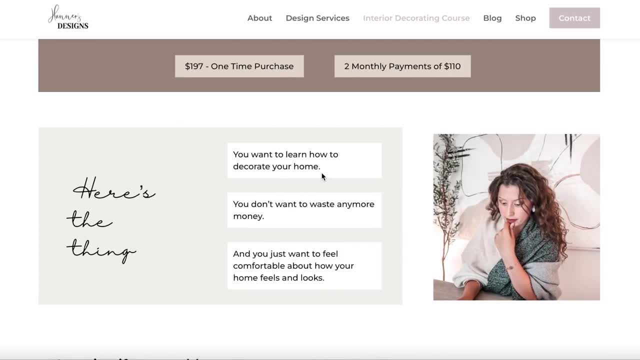 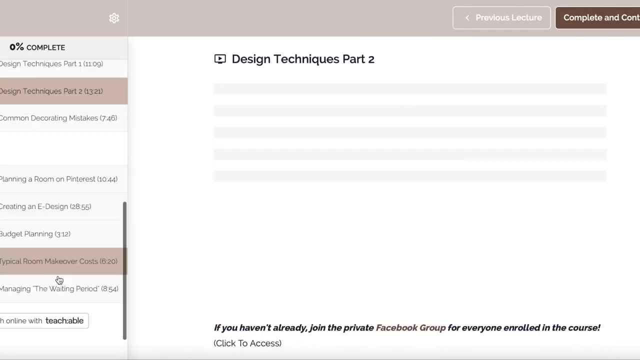 all by yourself- Well, with my help, of course. The course only takes out three hours total, and we'll walk you through everything a new or seasoned homeowner needs to know before wasting any more money trying to decorate, because we have all the best home design tips for you. 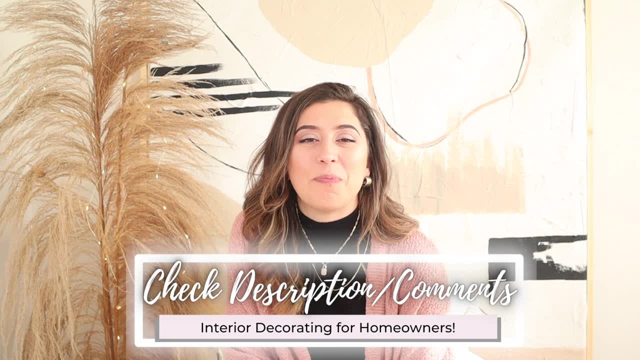 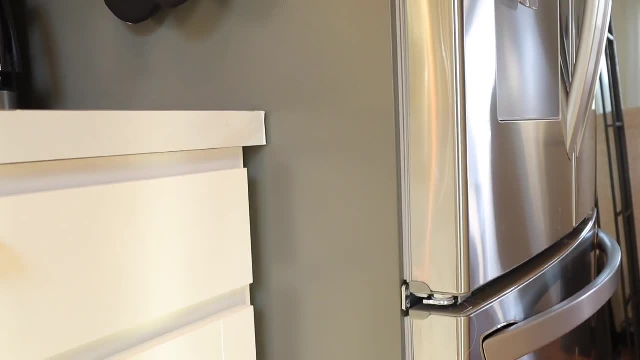 Make sure you click the link in my description box and comment section. Back to the fridge organization tips. Tip number nine is to check if you have a counter-depth fridge or not. We do not have a counter-depth fridge and after testing these bins in the fridge, 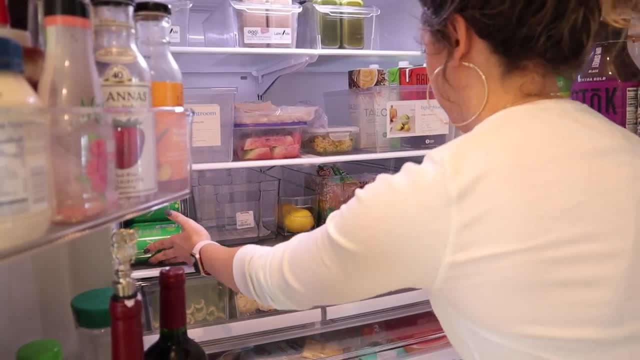 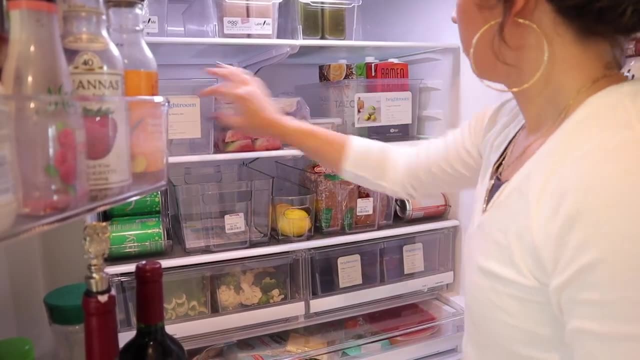 they were more shallow than I thought, and so we probably could have been fine going with a counter-depth fridge. However, I did look it up and saw they tend to be a bit more expensive, so I'm totally fine with there being extra space behind our bins if we ever needed it. 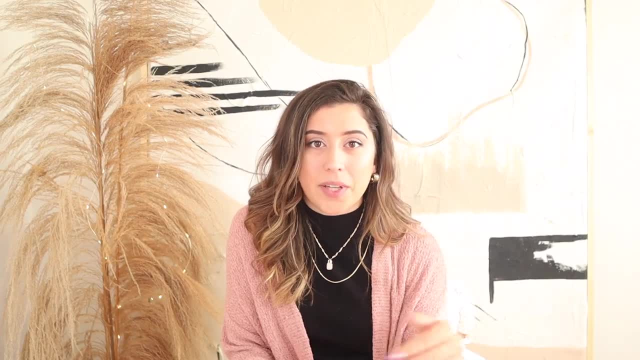 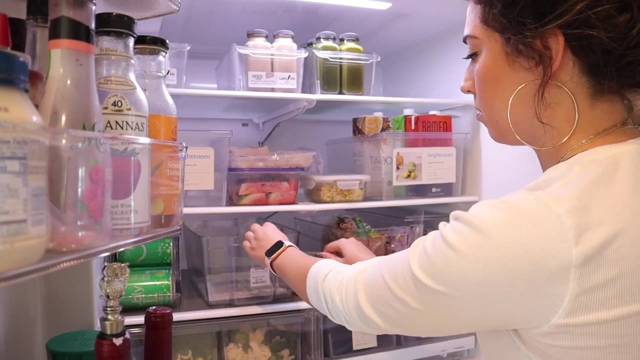 or we can push the bins further back and have space in front of the bins again If needed. Which leads me to tip number ten, which I learned from the home edit book. and it's okay to push your items to the front and have unused space behind them if that's going to. 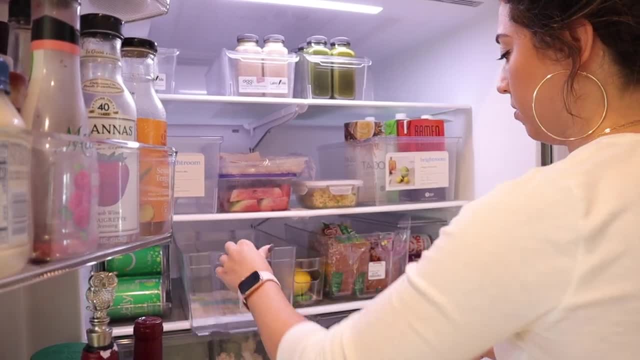 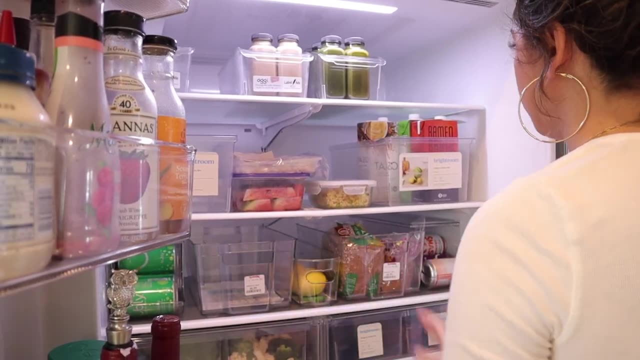 keep you more organized because you can see everything And, honestly, that has worked wonders for our pantry spice organization, which I have a video on that one too, if you missed it. Overall, the concept is that you don't need to move things around to see what's behind. Instead, it's all in. 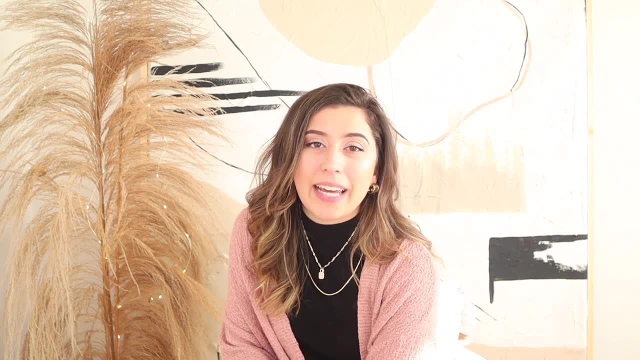 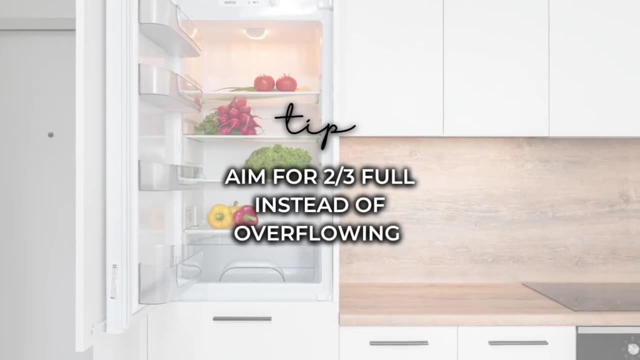 the front and there's nothing hidden. As I was playing around with the bin layout, things got a bit tricky as the bins were rubbing against one another. So tip number eleven is to aim for a two-thirds full fridge instead of a full full fridge. I don't know how possible that is for 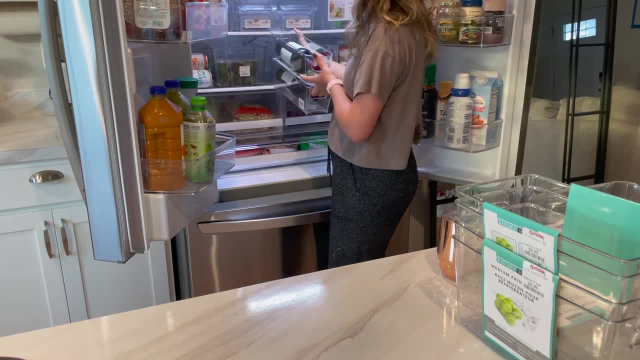 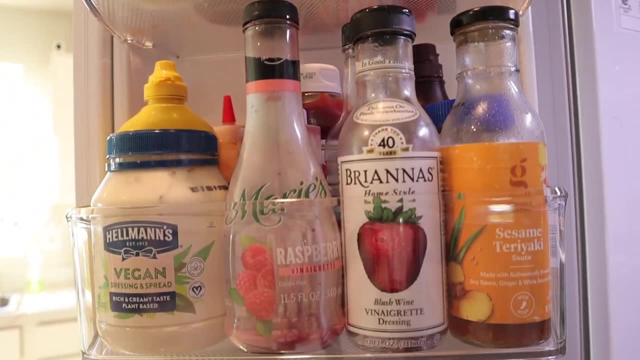 most people because we all have different fridge sizes. maybe we have a lot of people in the house and sauces are taking up like 53% of the fridge, okay, So comment down below if your fridge has been commandeered by sauces like ours has. I swear our fridge is mostly liquid. Tip number: 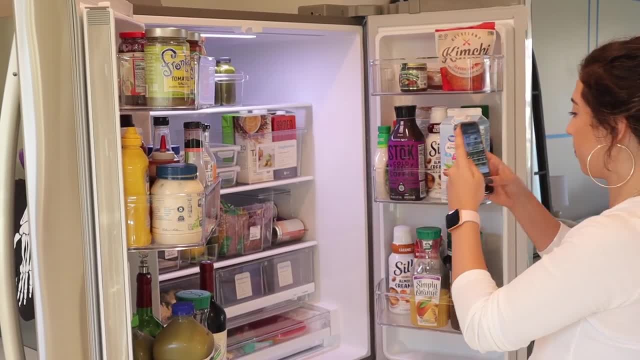 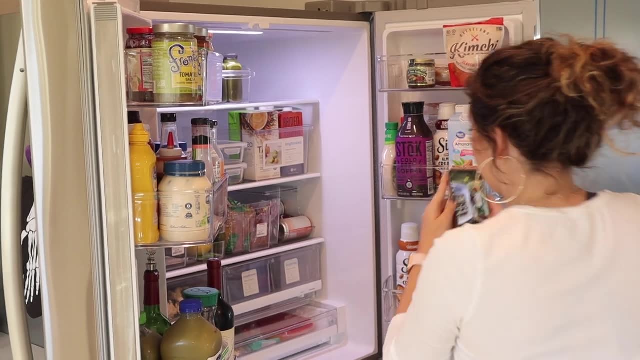 twelve is to take a picture of your fridge after you've done your first round of bin organizing, because you're going to want to stand there with the doors open thinking is this the best way to organize this? And while you're sitting there contemplating life, you're letting all the cold. 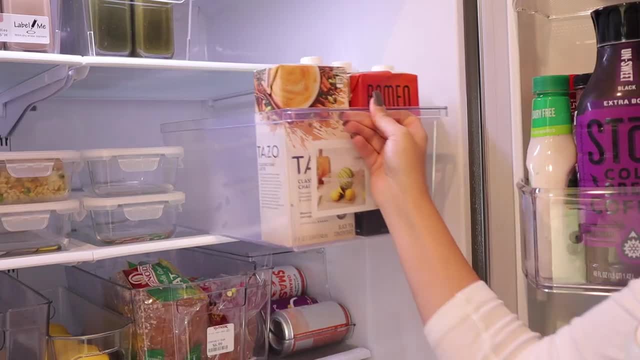 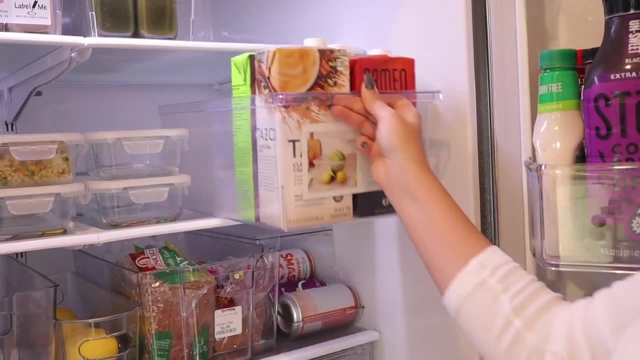 out, air out and, like my dad would say, you're burning money. Tip number thirteen is to have a free-for-all spot in your fridge for things that may not work in the tidy system you've created. Think of it like a catch-all. After using my fridge for a couple of weeks, I decided on a. 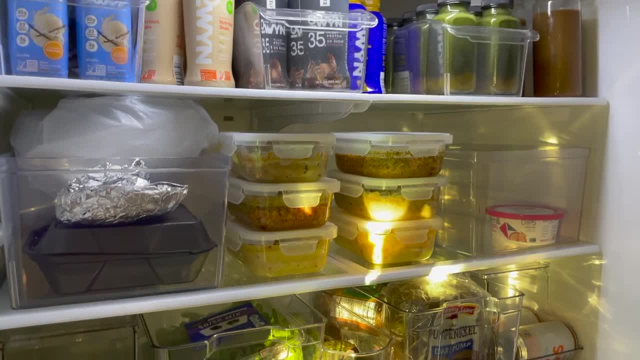 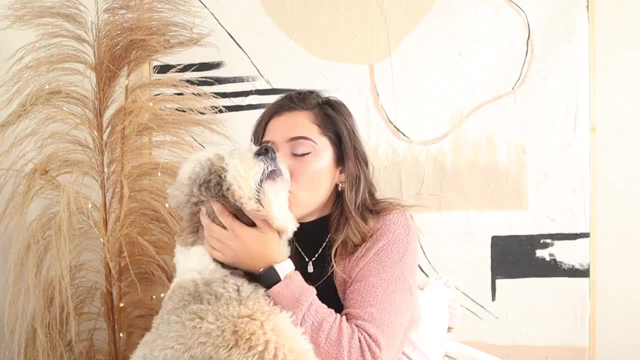 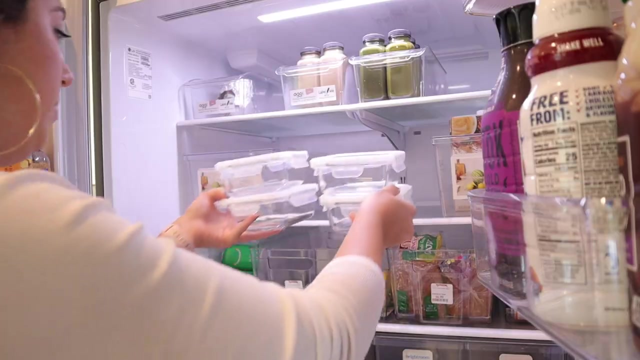 spot that I felt like would work for us. It's also a backup spot when the fridge doors are full. Tip number fourteen, which is probably going to catch you off guard, is to store your empty meal prep containers in the fridge. Tip number fourteen is to store your 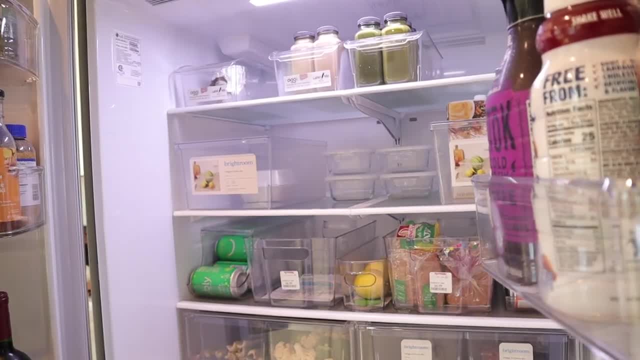 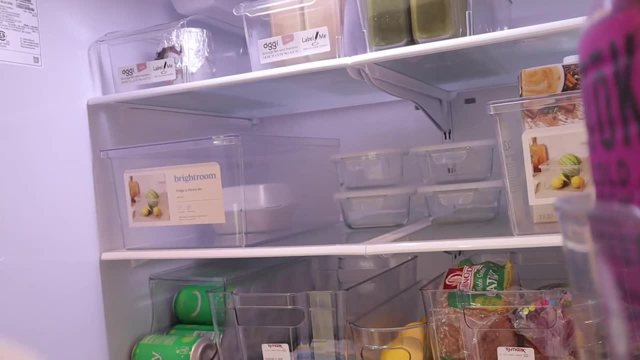 empty meal prep containers in the fridge. This will remind you to cook and replenish your food for the week and in general, you don't need to store them and take up other kitchen space when the containers are going to be in the fridge either way. Radical idea, I know, but so far. 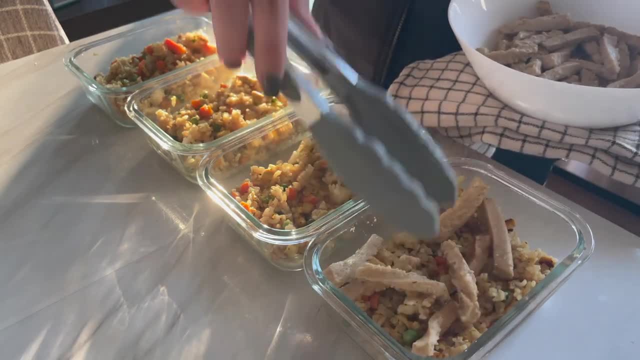 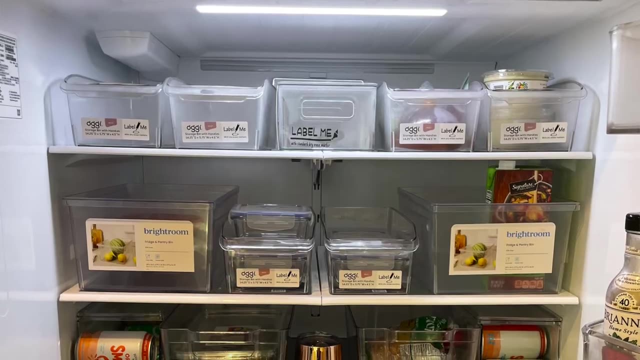 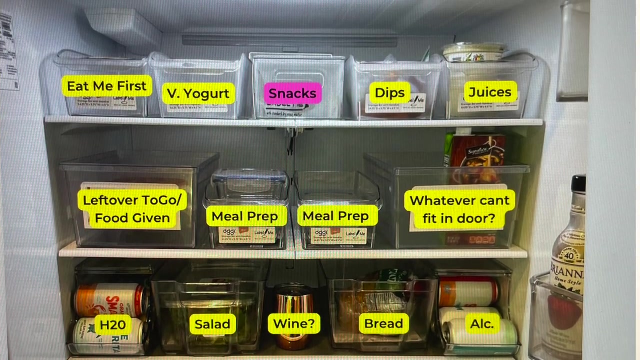 so good for us. It also discourages anyone from using that space that you've dedicated for your meal prep containers and therefore they act as placeholders. Tip number fifteen is to plan your fridge organization virtually. I use Canva for all my eDesign projects, which I'll link down below for you. It's easy to use. I use it for everything. 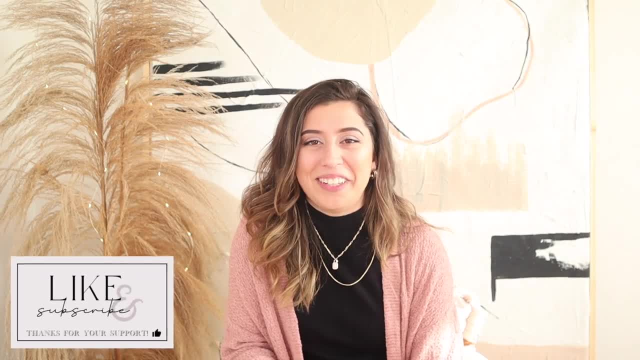 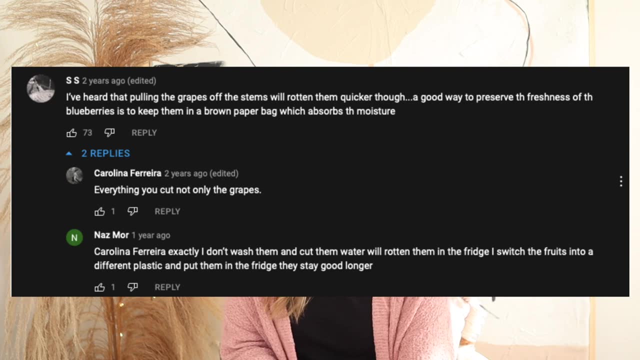 in my life and business now, including organizing my fridge. apparently, Tip number sixteen, which I learned from well people right here on YouTube, is that there are rules regarding your produce fresh in the fridge or surprise out of the fridge. I saw so many comments on. 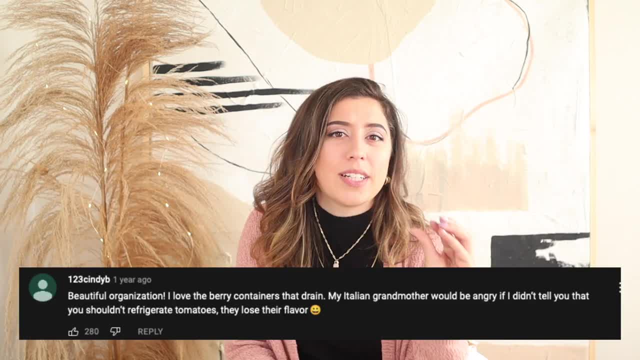 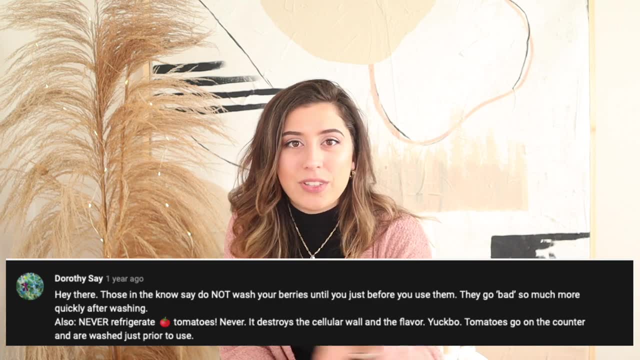 other fridge organization videos saying tomatoes don't belong in the fridge because they lose nutrients and or flavor, along with uncut onions, those belong in a dark, cool area. or even: don't wash or cut your fruits and veggies days prior to consuming, because they spoil faster that way. 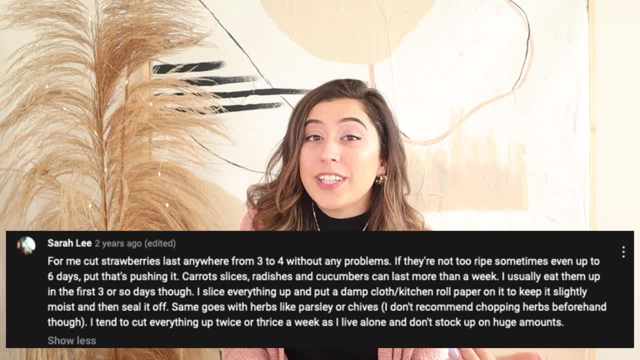 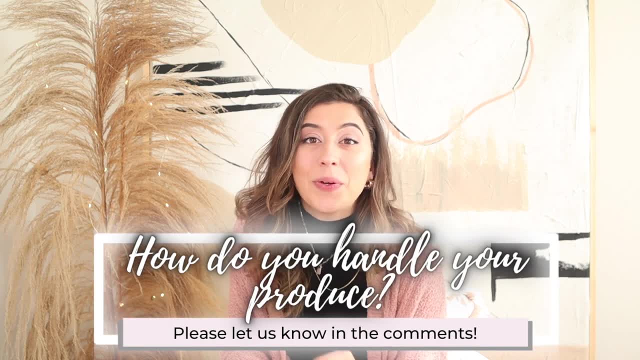 etc. Many people recommended exploring which foods should be in the fridge and which ones are better left in the pantry, and not only with that, but how they should be handled. So question for you is: how do you handle your typical produce when you bring it home, and how has those methods worked? 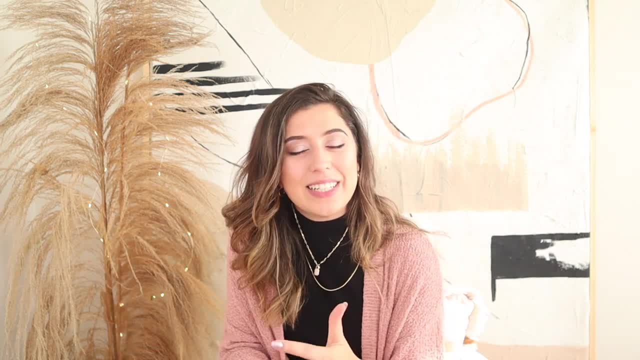 for you. Tip number fifteen is to plan your fridge organization virtually. I use Canva for all my fridge organizations videos, so please let us know down in the comments. I think it's going to take some trial and error to figure out what lasts best and under certain methods, but here's what I've. 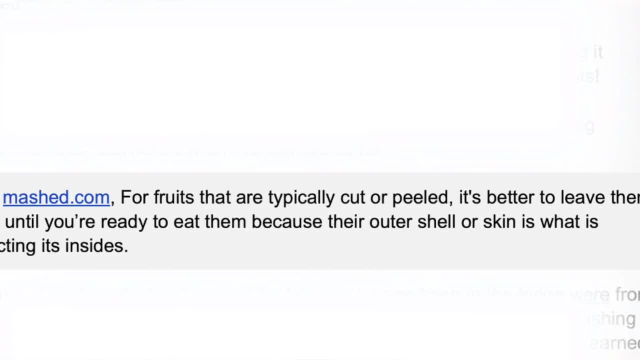 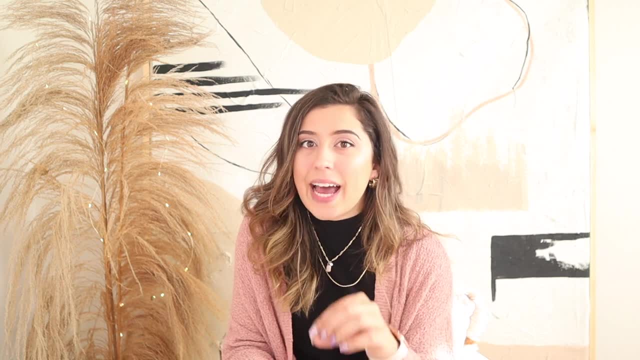 learned so far From mashcom. for fruits that are typically cut or peeled, it's better to leave them uncut until you're ready to eat them, because that outer shell or skin is actually protecting its insides. And one of my favorite tips I learned about keeping berries fresh in the fridge was